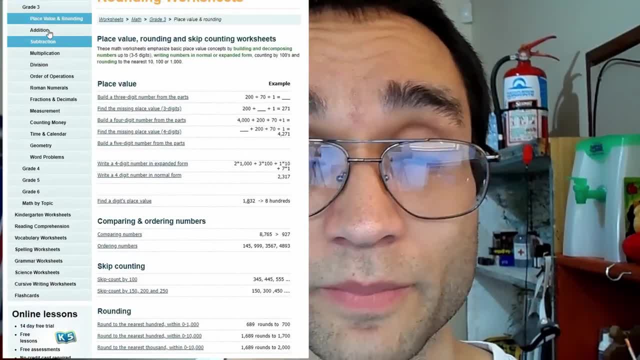 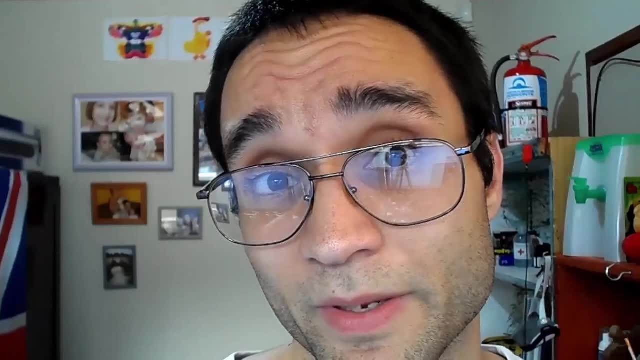 different topics. It's so many different topics I don't even need to do them all. We can skip over some of those worksheets. Also, they give you five different versions or six different versions of each worksheet normally, which is great because it means you can repeat them again later. 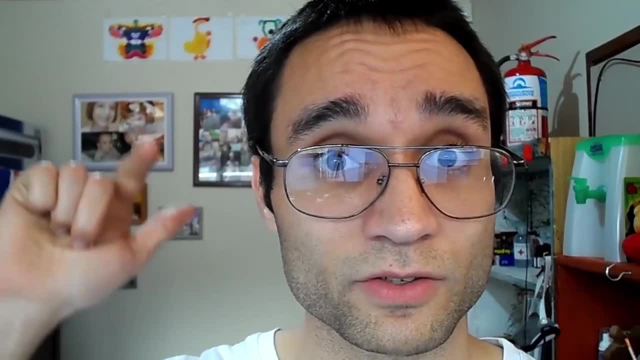 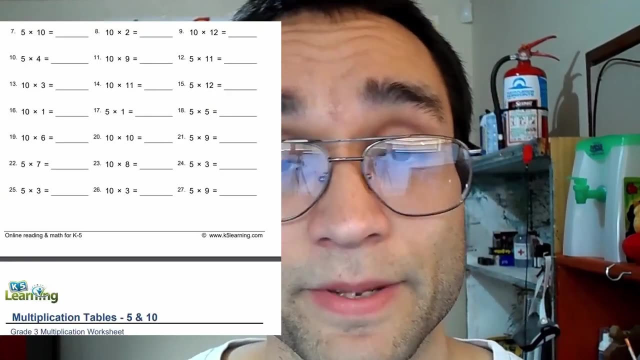 Okay about this website is it does give you kindergarten to grade six, which is great for the lower level. I use it for British students, international students and American students, but it is a bit drill and kill. It does have just huge worksheets with loads and loads of exercises. 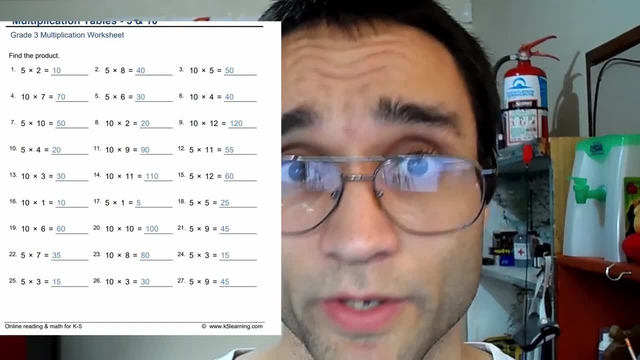 and sometimes that's really really good. Sometimes, especially younger kids, they just want to do that. They just want to sit down and do loads of multiplication, loads of addition. They want to get an idea and just do it again and again, and again. 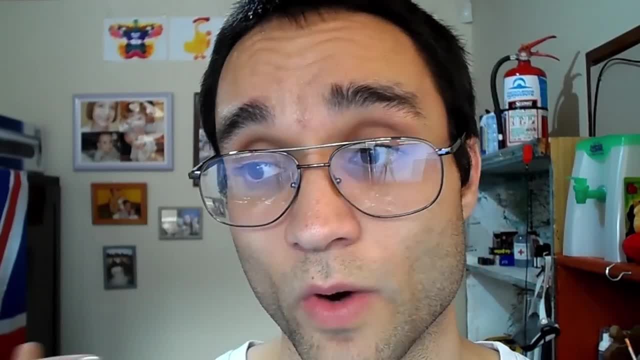 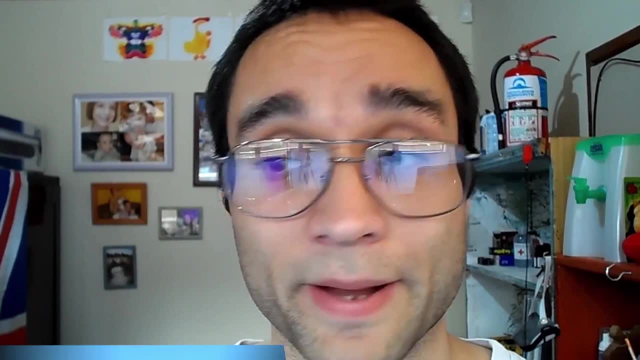 They want to do it every day, but they do want to do it sometimes, So I do use that quite a lot And it was a really good lifesaver when I started out. Okay, after that we have Corbett Maths. Corbett Maths Primary is really, really good for elementary school and primary school. 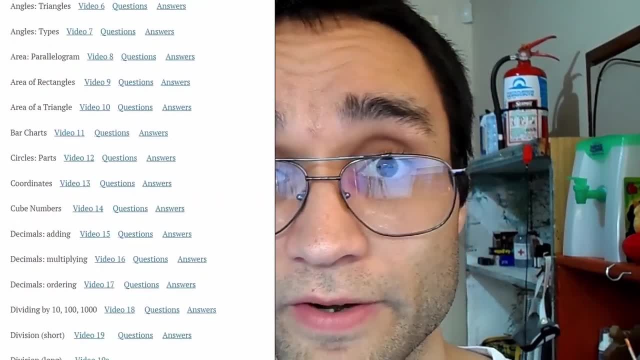 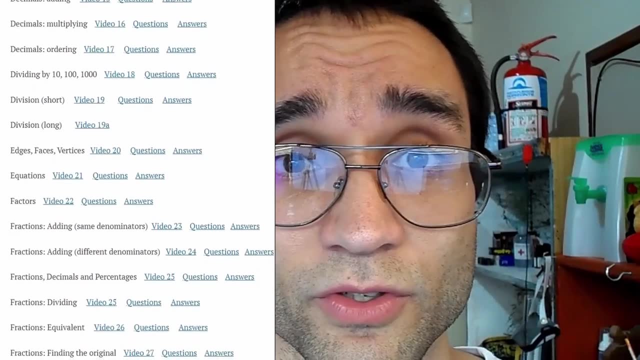 It doesn't give you the structure. It gives you a whole list of PDFs which are very, very good. It also gives you all the solutions and there's videos on each one as well. I never use the videos, I never use the solutions, I just use the PDFs. they're really, really good quality. They're a 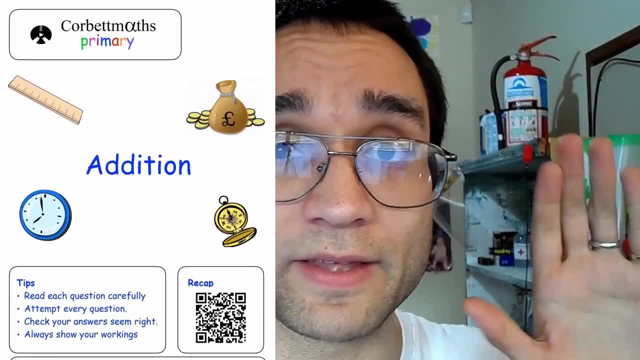 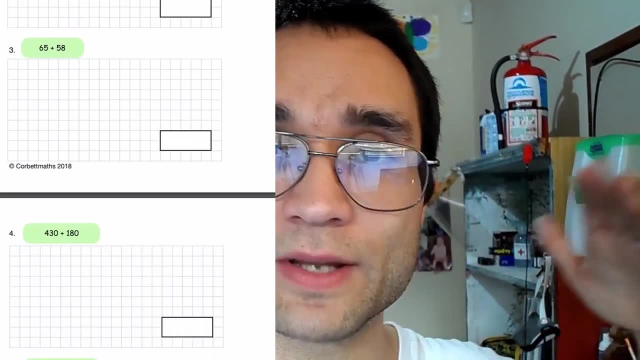 very nice mixture of questions, mathematical questions and then word questions, math questions and word questions in the same PDF And they take an idea and it's very graduated, so it's very nice. They take it from about second grade, third grade or year two, year three. 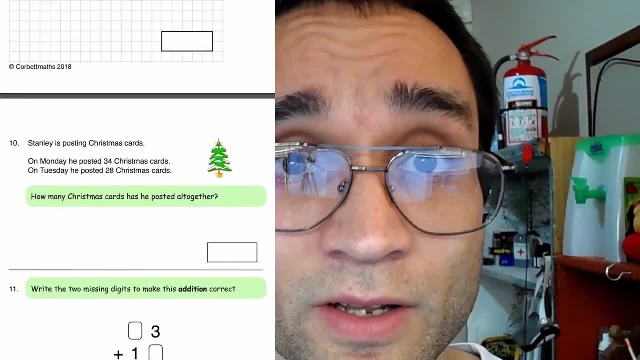 up until a year, six or sixth grade. So it does give a lot of information. It does give a lot of knowledge to you. It does give you a little bit of information as to what this is all about, get quite difficult towards the end, but it does give you this really differentiated and graduated. 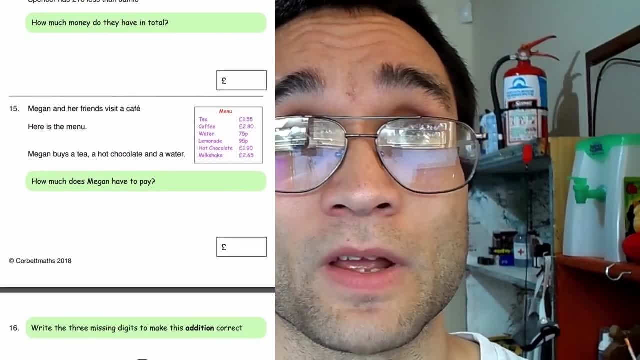 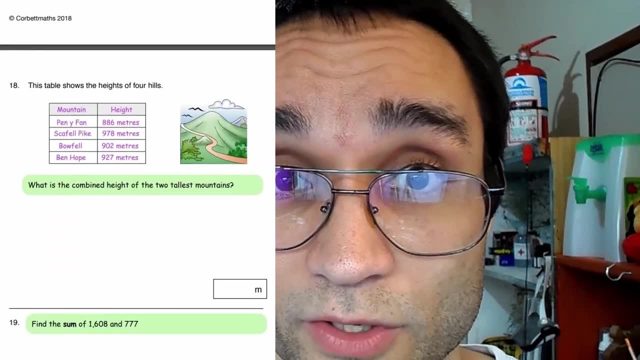 worksheet, which means you can pick it and use it for any student. um, the problem with that is that you can't use it more than once. you can use it one time or two times and the student will finish it. so you need a bit more long-term solution, a longer term solution, for than this, but it's really really. 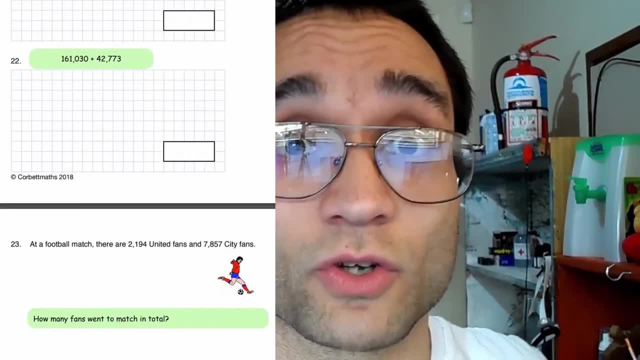 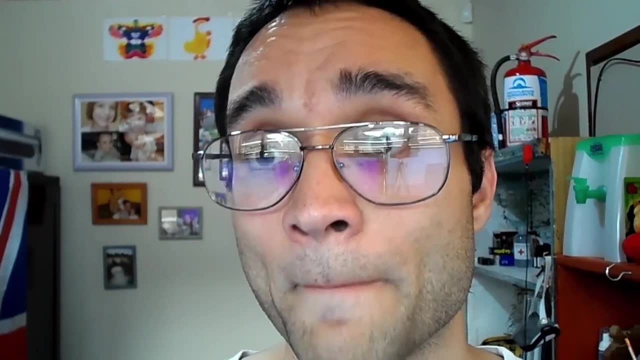 nice quality. you love it. my students love it as well. they really like that mixture of questions and then word questions, um. so it has a whole bunch of different topics. on the core bit, primary maths, it's really good. after that we go to secondary and um the my i use this more than 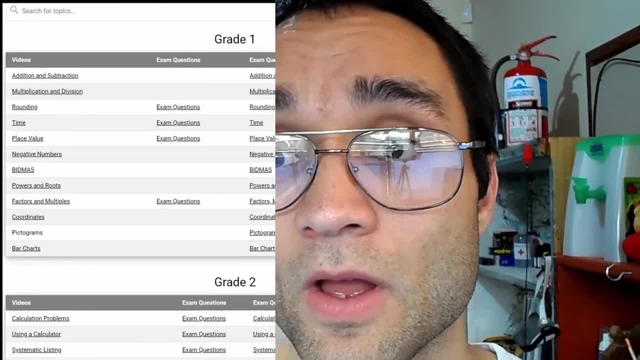 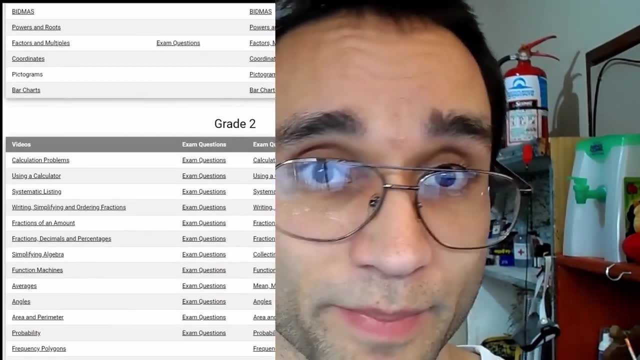 anything is the british education system. i use um mathgeniecouk. i also use this for the american education system, but it takes um individual topics and explains them. but the really good thing about this is it has a lot of structure to it and it goes from the easiest level right down to the 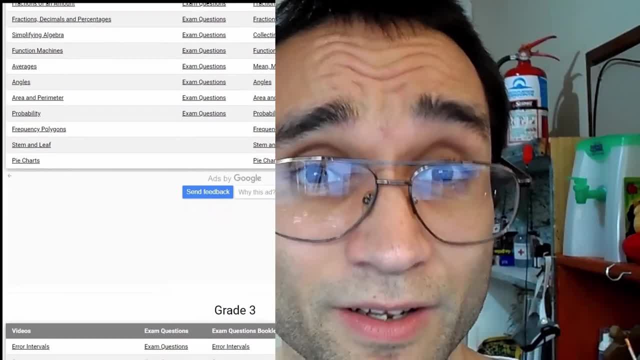 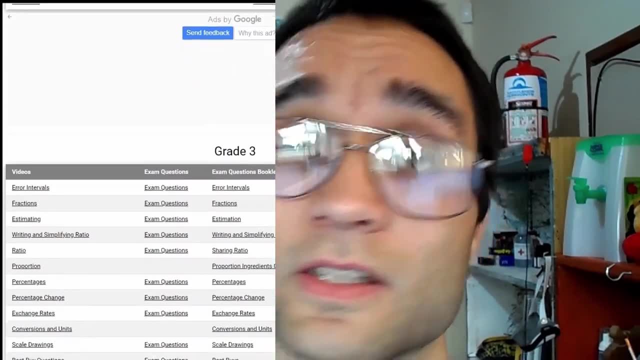 most complicated level, so it goes from about year seven up until year 10, which is like grade seven up until grade 10, and so i can use it to do a couple of different things, and if i know that i need a subject, i can just go to the curriculum and i can go to the curriculum, and i can go to the curriculum. 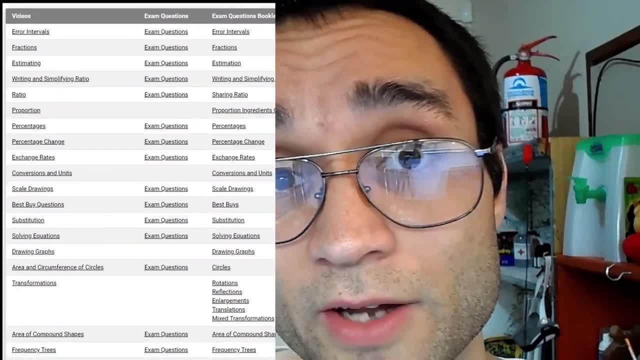 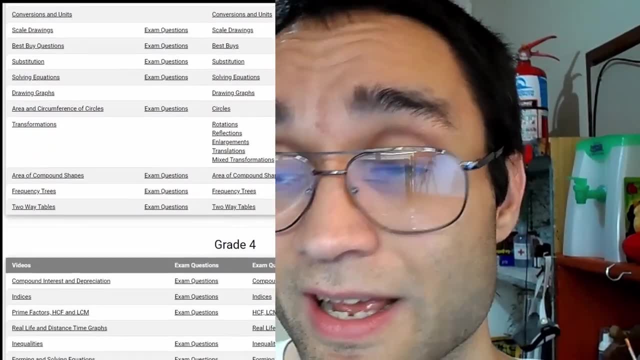 and i can go straight into that. if i know my students need something like trigonometry, i can find it very quickly. we can go straight into that. if i don't know what to give them or they're working for a long period of time, we start at beginning and then we go right down to the end. 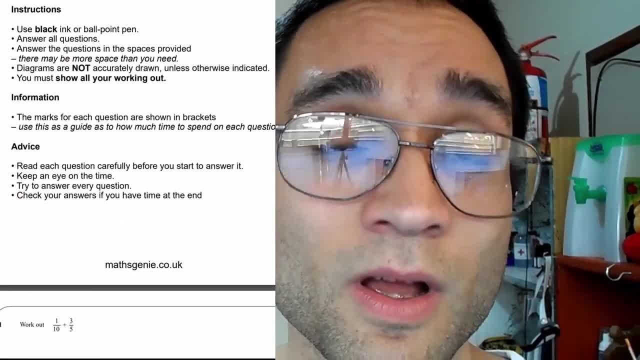 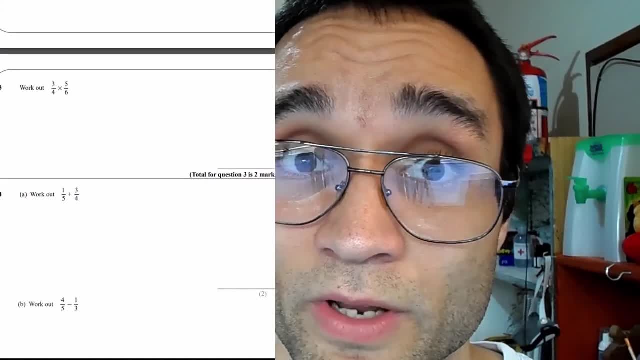 and like that i can be sure i cover every single topic in the curriculum, which is great. it's really really detailed, really high quality. the question packs take about an hour- 30 minutes to an hour for each one, depends on your student. students take a full hour to do one, which is just right. it's perfect, it's. 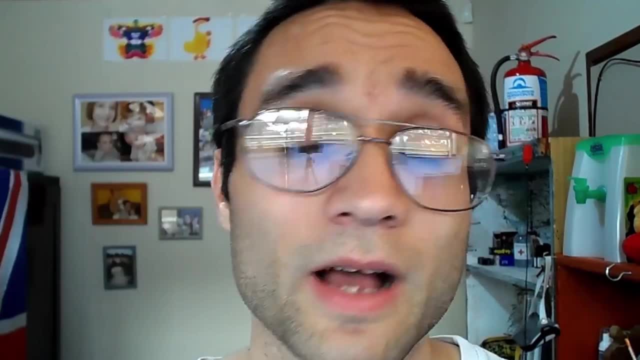 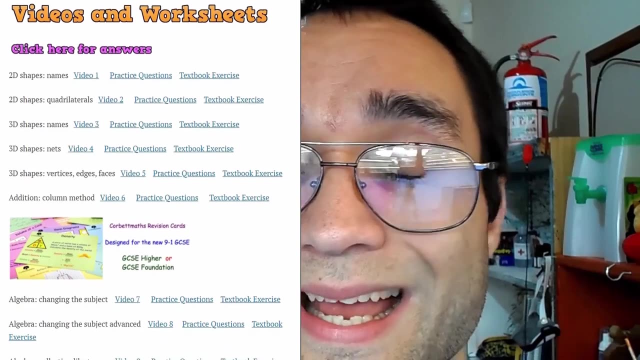 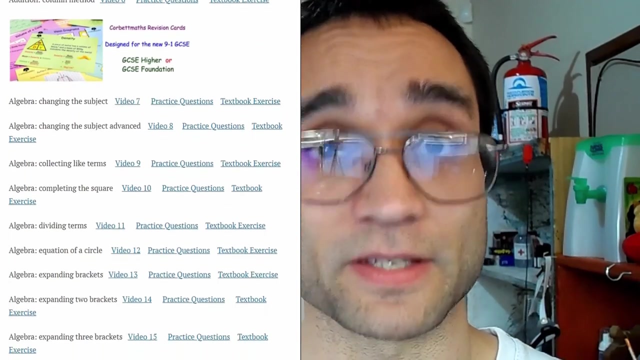 really nice. I use that more than anything else. again, I'm gonna use Corbett maths for secondary school level. Corbett maths also has a secondary school level for mathematics worksheets and we're gonna work through them in the same kind of way. that doesn't have the structure. it doesn't have this there's. 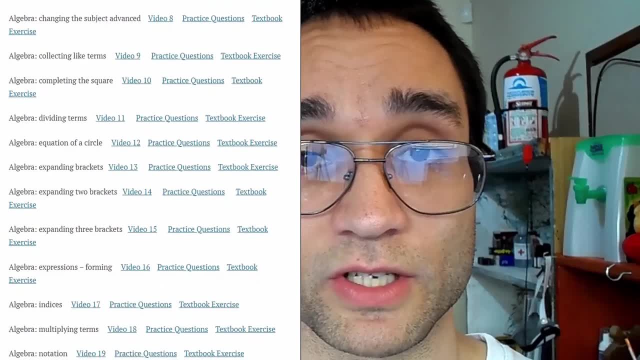 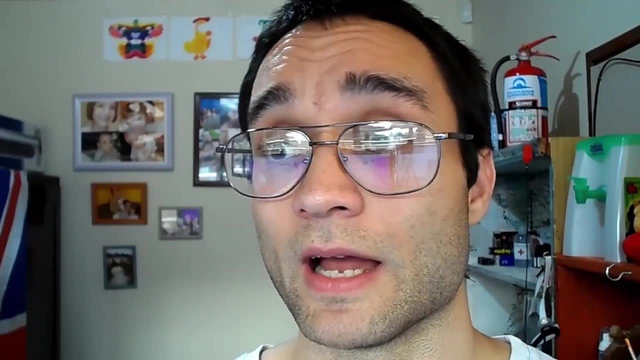 this easy to look, complicated structure. it just has a whole bunch of worksheets which are alphabetically organized, so you need to know what you're teaching. you can find it very quickly, but then you do need to add that structure. when I'm teaching American students, I'm going to use cutter software. now cut the. 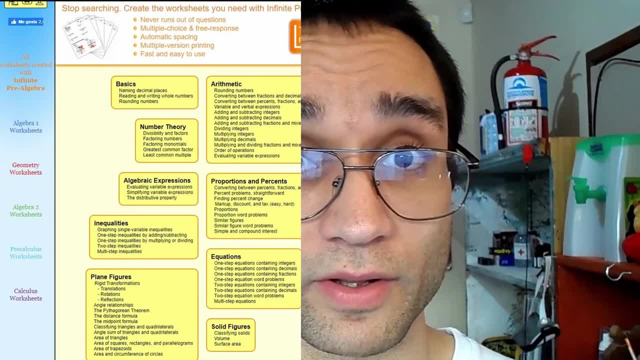 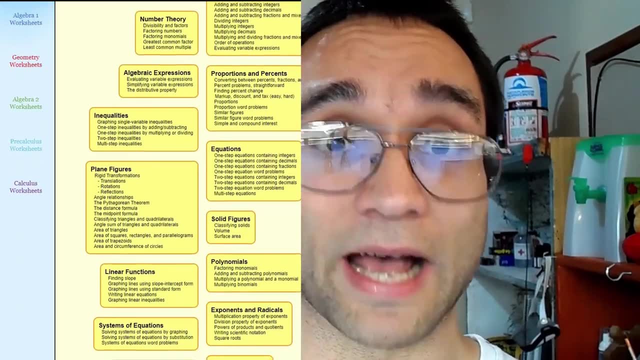 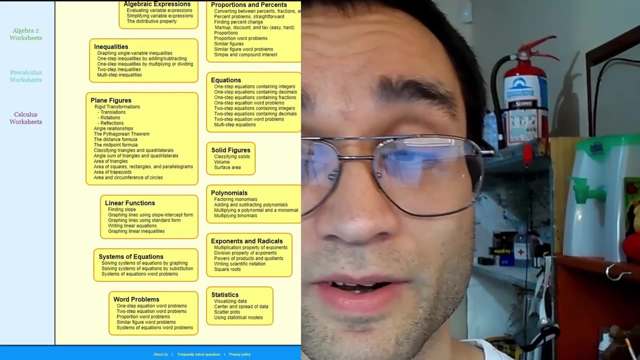 software is really good software, really really nice. it's based around the core, the common core, as that's great. it has a pre algebra for seventh grade students: algebra one, geometry one. algebra two, pre calculus and calculus. I'm gonna fingers that one and that's really really cool. it means: